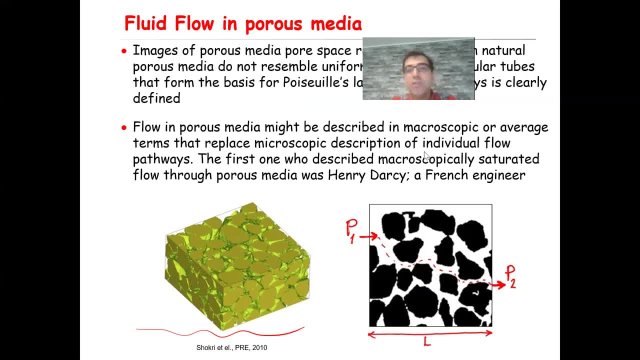 that replace the microscopic description of individual flow path phase. I'd like here to highlight that, of course, now that there are several methods, for example numerical methods, that can be used to describe flow through each individual path phase and pores like I don't know, direct numerical simulation, lattice Boltzmann simulation and so on, 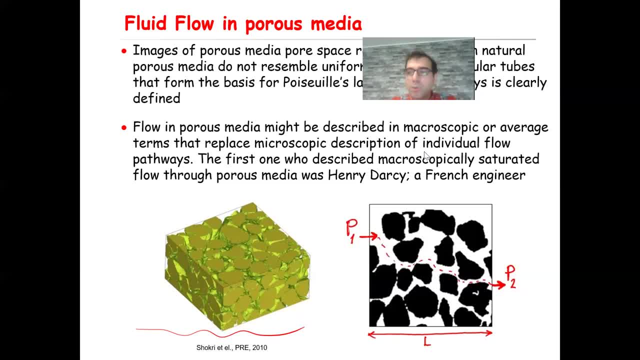 And we actually use some of these methods in our current research. But obviously discussing about the details of those methods are beyond the scope of this bachelor level groundwater hydrology. So here in this course we focus only on a macroscopic description of the flow through porous media. 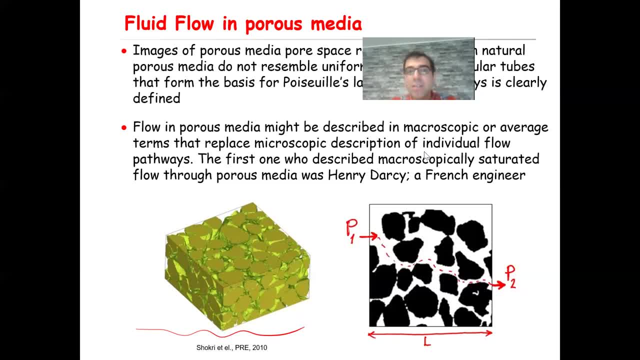 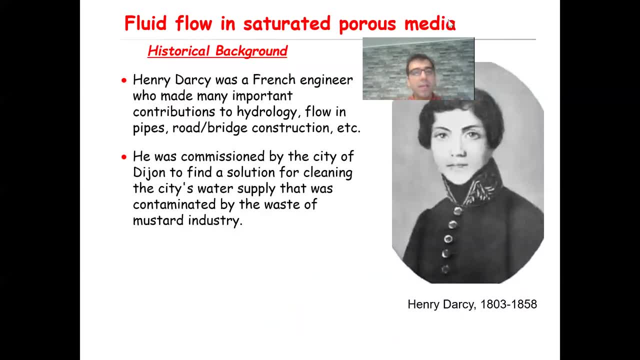 And the first one who described macroscopically saturated flow through porous media was Henry Dorsey, who was a French engineer. OK, A little bit of history here. That is, Henry Dorsey was a French engineer who made many important contributions to hydrology. 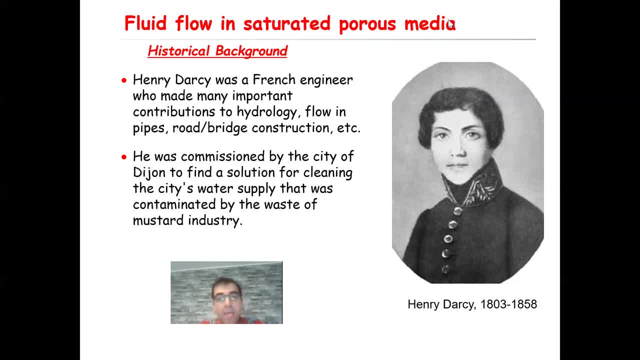 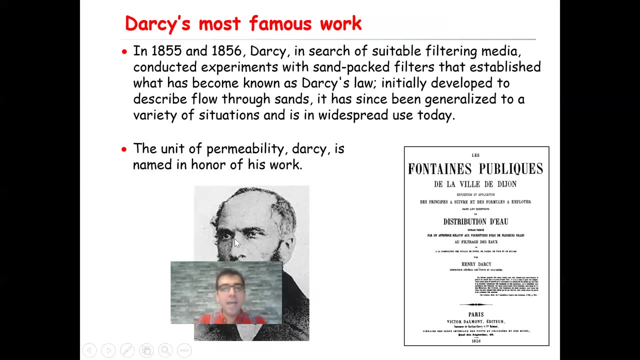 flowing pipes, road and bridge construction, etc. He was commissioned by the city of Dijon, which is in France, to find a solution for cleaning the city's water supply that was contaminated by the waste of mustard industry. OK, In 18,. let me move this one here. 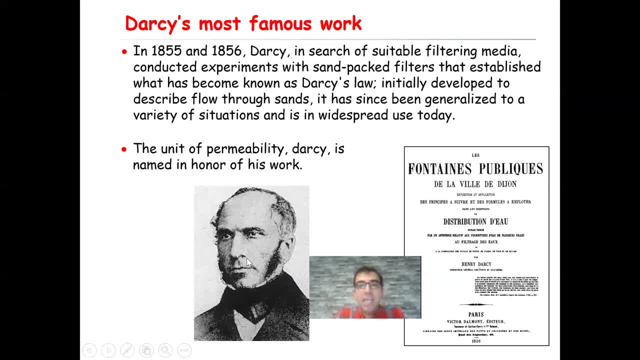 In 1855 and 1856, Dorsey, in search of suitable filtering media, conducted experiments with sand packed filters. OK, That established what has become known as Dorsey's law. Initially, that law was developed to describe flow through sands. 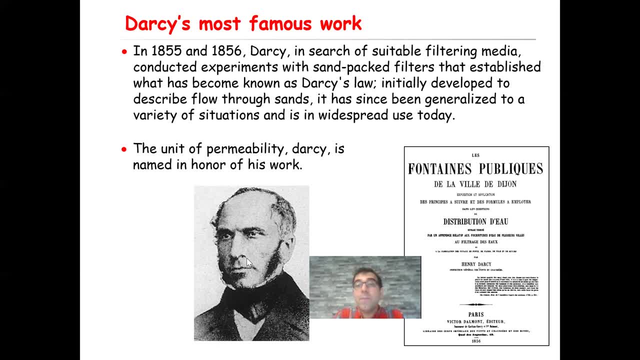 And it has since been generalized to a variety of situations and is in widespread use today. Basically, he was testing different sanding materials to find a suitable filter for cleaning of the water supply of the city of Dijon, And in those experiments he basically found the law. 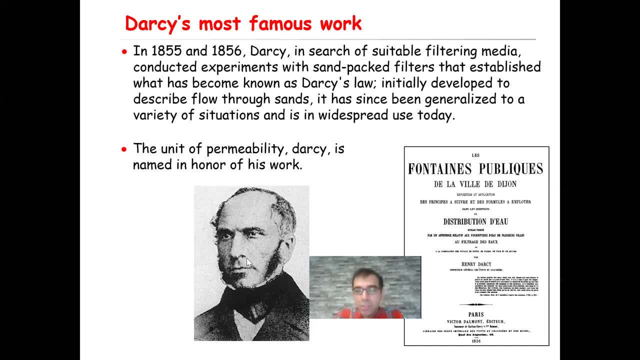 the relationship that has become known as Dorsey's law And the unit of permeability, which you will learn about permeability in a few minutes. Dorsey is named in honor of his work. OK, So basically that was his experimental setup. 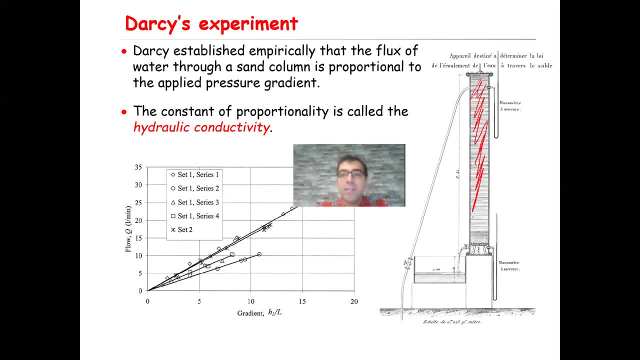 He had this big tank here, You see this one. He filled it with a different type of sand, different type of. basically, he was looking for a proper filter, suitable filter, And you apply pressure here And then you collect the volume of the outflow at the bottom here. 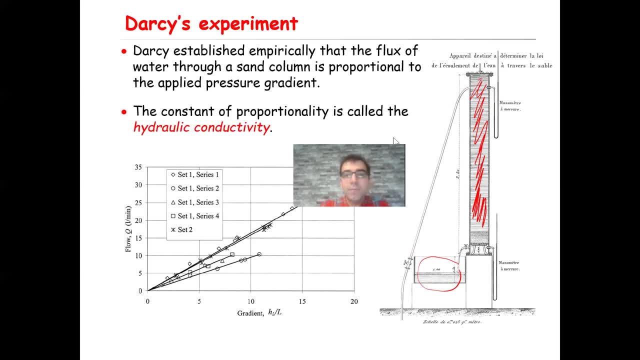 OK, And then let me move this one here. He found that if he plots the volumetric flow rate, the capital Q volumetric flow rate, versus the applied gradient pressure gradient, he gets a straight line. OK, And here different symbol, I guess, refers to the different filtering media. 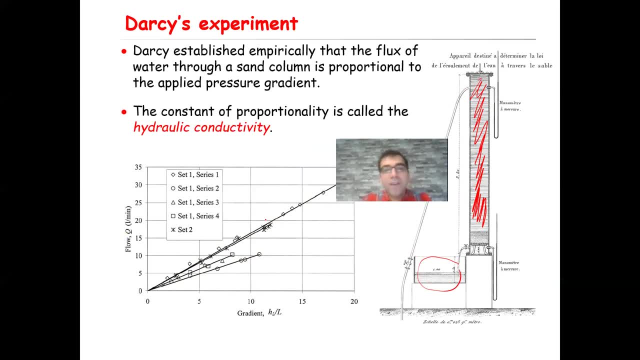 different type of sand, But in each case he found that he established empirically that the flux of the water through a sand column is linearly proportional to the applied pressure gradient, And the constant of that proportionality is called hydraulic conductivity. OK, 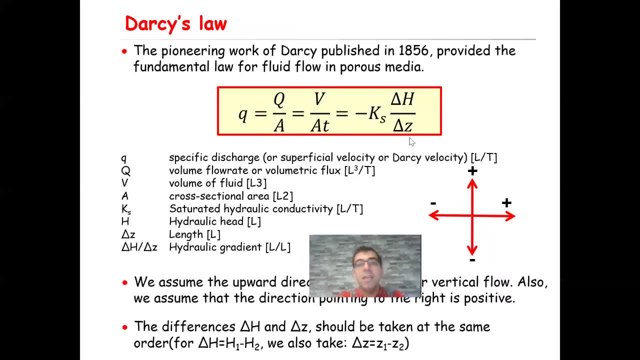 So Dorsey law is expressed as: Q, that is the Dorsey velocity, equal to Q capital. Q, That is volumetric flow rate divided by the cross-section of the column. basically, And volumetric flow rate. you can calculate it as V. 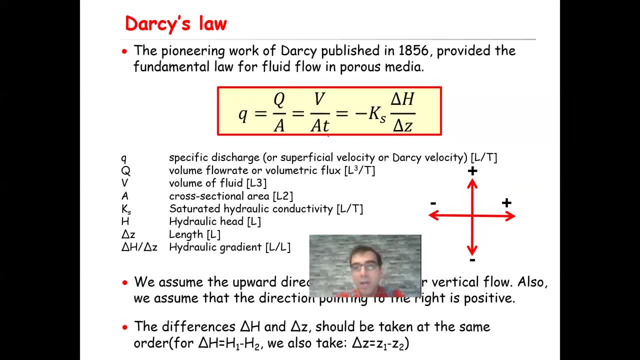 that is the volume of the collected water divided by time times. A. OK, And Dorsey's experiment found that this volumetric flow rate is proportional to the applied hydraulic, basically gradient, And the constant of that proportionality is called hydraulic conductivity. 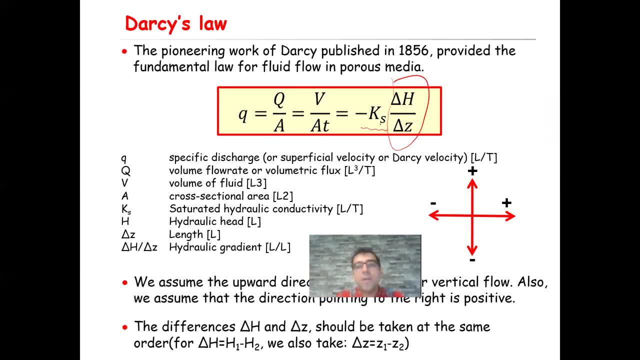 saturated hydraulic conductivity here, because you are dealing with saturated flow Ks. OK, So then, since this is, H is hydraulic head with the dimension of length and delta Z is the length. therefore, delta H over delta Z is dimensionless here. 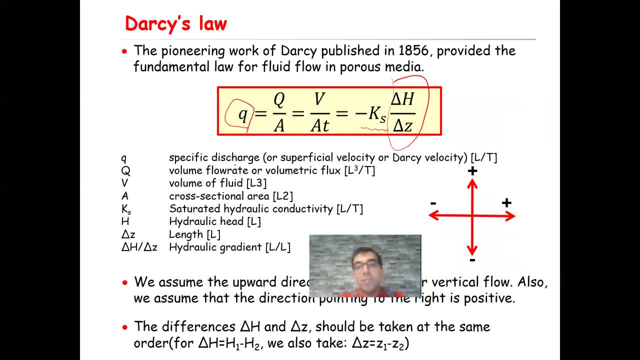 And the Q, the Dorsey velocity, or sometimes called a specific discharge or superficial velocity or Dorsey velocity, has the dimension of length per time that is like velocity. Therefore Ks saturated hydraulic conductivity has the unit of velocity. 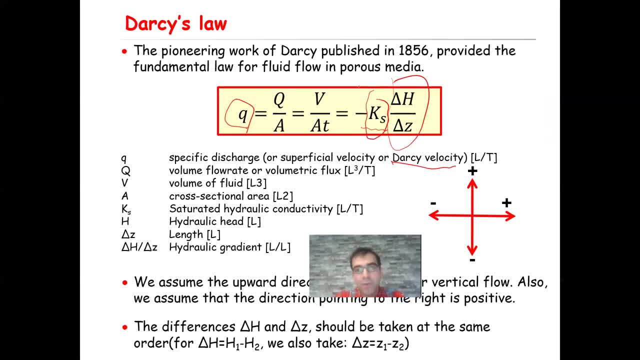 the same unit as velocity, that is dimension of length per time. OK, Here, in this course as well, we assume the upward direction is positive. OK, In this course, we always assume upward direction is positive And also direction. 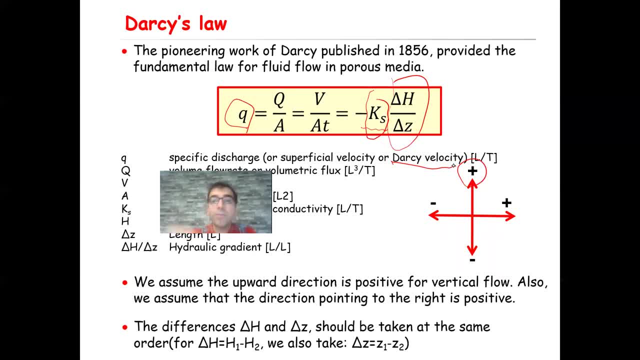 yeah, upward direction is positive for vertical flow, And also direction pointing to the right is positive, OK, And direction pointing to the left is negative, And the downward flow as well is negative. Another thing that you need to consider here is that the differences 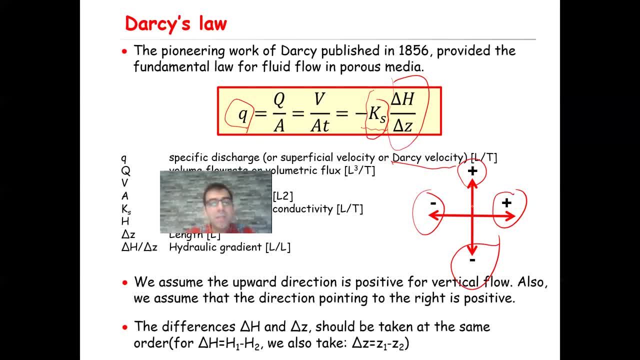 delta H and delta Z should be taken at the same order. What does it mean? It means, for example, if you write delta H is equal to H1 minus H2, you should follow the same order. Delta Z will be Z1 minus Z2.. 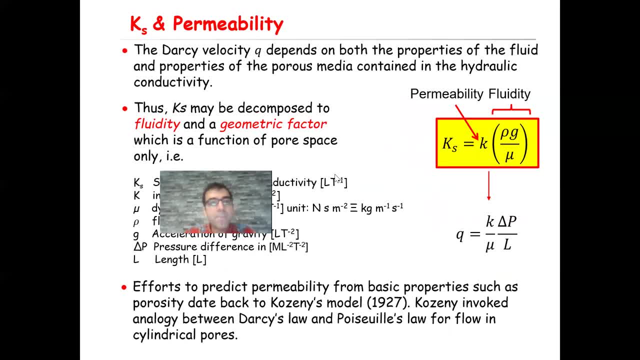 OK, So here, so, as you can imagine, if you, for example, let's say, use water, use another type of fluid, I don't know, let's say honey, for example. right, Depending on the type of the fluid that is flowing through your porous media. 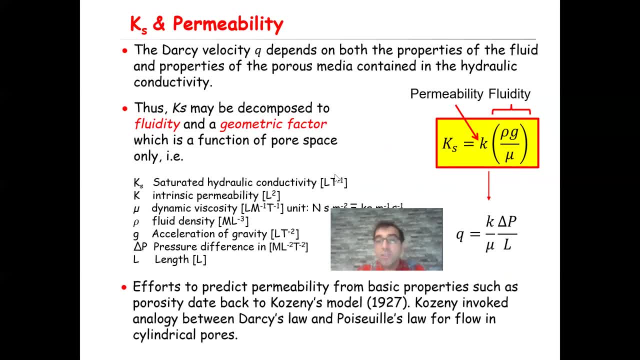 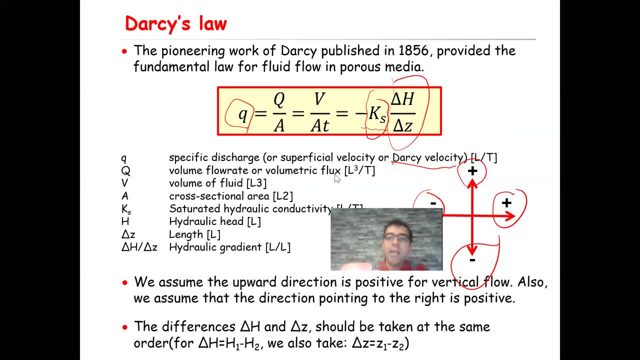 or even, or, for example, when you change your porous material. so when you change the fluid or change the porous material, you can imagine that the velocity will be different. right, But when you look at this equation here, this is the velocity Q and delta H over delta Z is dimensionless. 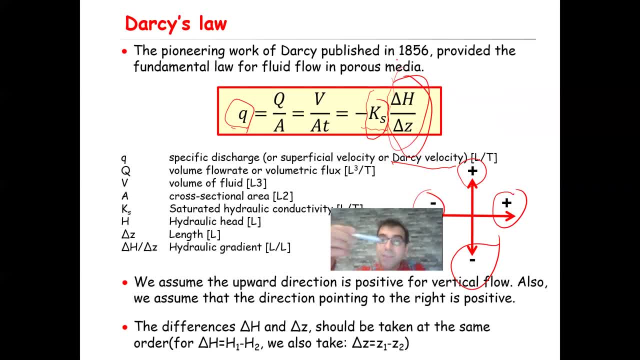 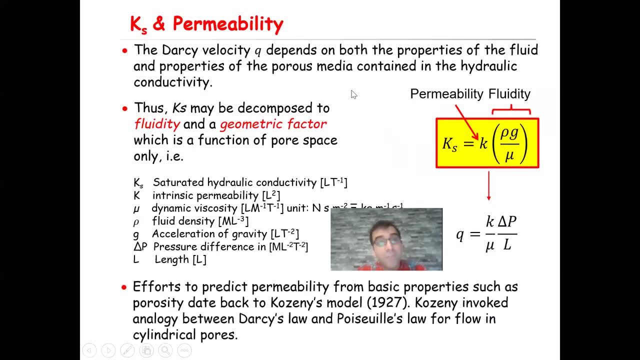 which is the hydraulic gradient. Therefore, these effects of the fluid properties and the effect of the porous media properties on the flow should be contained, or is contained, in the saturated hydraulic conductivity. OK, So the Darcy velocity Q depends on both The properties of the fluid and properties of porous media. 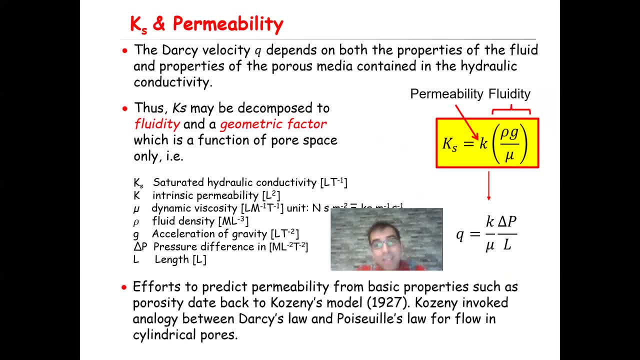 contained in the hydraulic conductivity. Therefore, the Ks, the saturated hydraulic conductivity, may be decomposed to fluidity and a geometric factor which is a function of the basically transport properties of your porous media. OK, So Ks, here you can split it, decompose it to K. 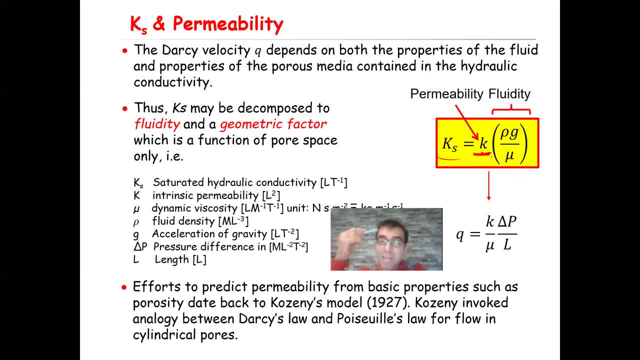 Let's call it permeability. It's called permeability that is related to the transport properties of your porous media, and another factor, rho G divided by mu, which is the fluidity which represents the fluid properties. Like here, if this is density: 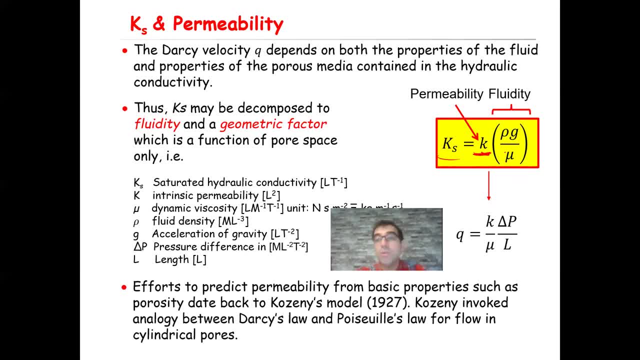 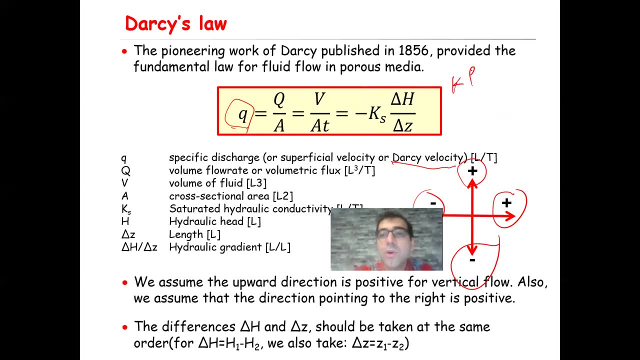 rho is density, G is the acceleration of gravity and mu is the viscosity. OK, So now if you write this equation here, Ks here, let me delete this one. So if instead of Ks I write K times rho, G divided by mu, 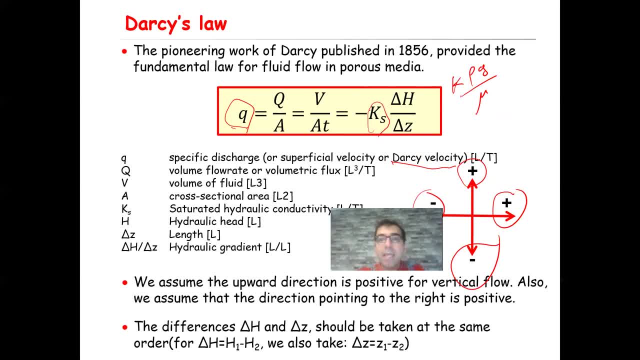 right. So here you will have instead of K, if I write K, that is the. this is the K, lower lower case K, that is permeability. rho G divided by mu, So delta H times rho G, basically H is: 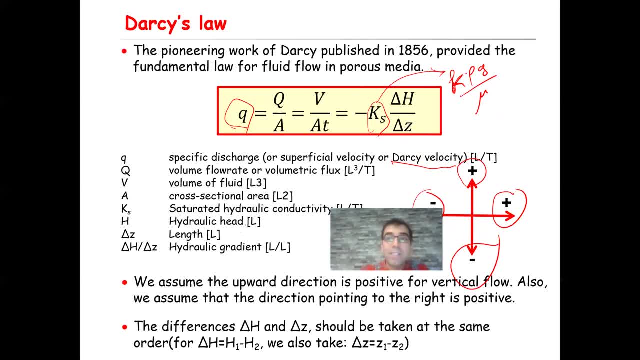 as mentioned here, it's a hydraulic head right. When it is multiplied by rho G, the energy is expressed in water potential. We had this discussion in the previous video in one of the previous videos, And so basically, H times rho G will be the potential energy expressed in basic water potential. 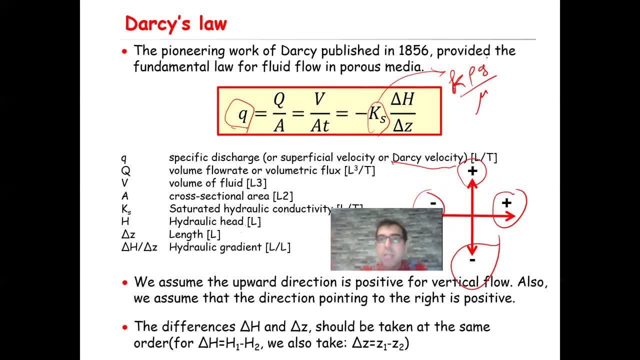 which will be the unit of pascal. OK, So instead of rho G, delta H, I can simply. instead of rho G, delta H, I can simply write delta P And then so here, instead of so, I write here delta P. 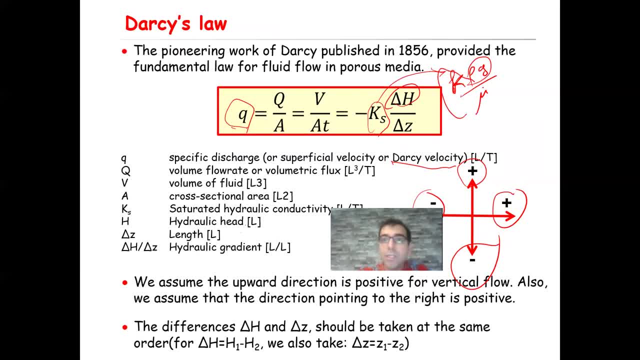 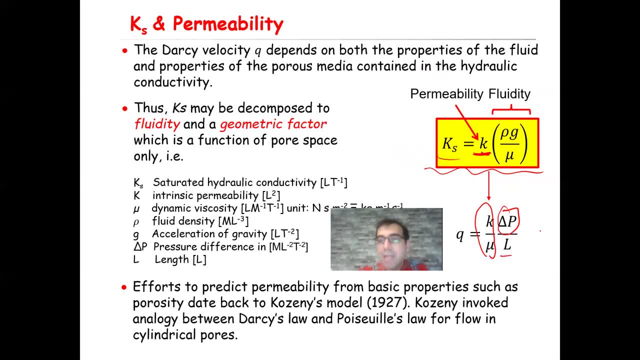 right, And then here you will have your K divided by mu, which is K divided by mu here, And then here, instead of delta Z I put here L, which is the length of the column, So you can basically write Darcy's law in this format as well. 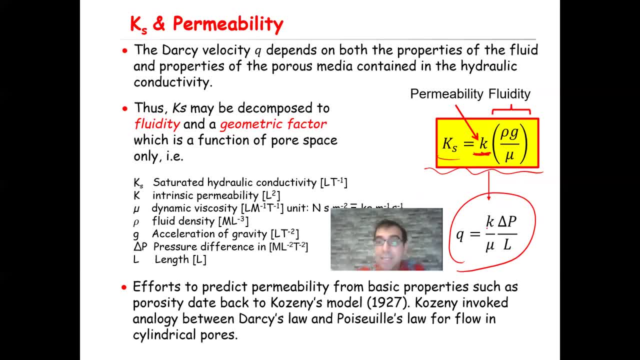 but pay attention here that K, the lower case K here is permeability, with the unit of length squared, And that unit you can obtain by a dimensional analysis of this equation, because you have the dimension of this one, you have the dimension of this density. 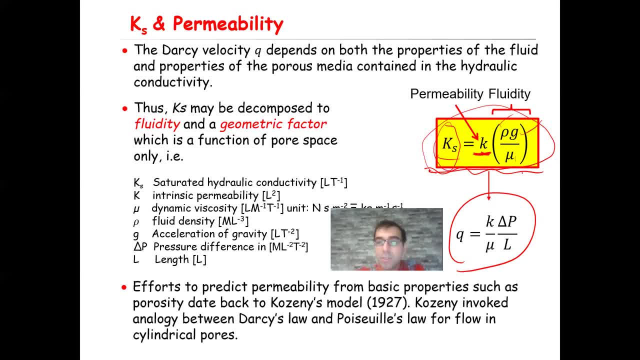 you have the dimension of gravity- acceleration of gravity- and you have the dimension of viscosity, And then you can calculate the dimension of the permeability. And if you do that, you will find the dimension of the permeability is length squared, as mentioned here. 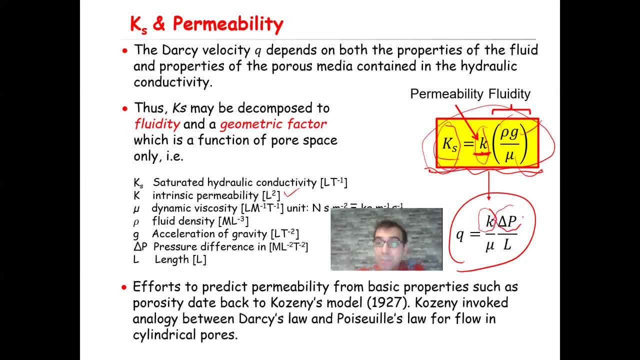 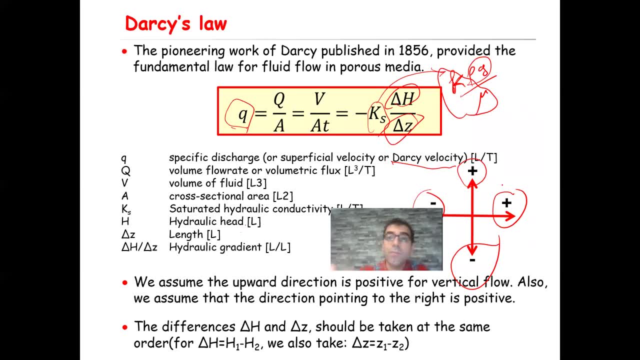 Okay, So the dimension of this is permeability, and here delta P is expressed in Pascal. Okay, And, and while here in this format the capital K is the is a hydraulic, saturated hydraulic conductivity with the dimension of length per time. 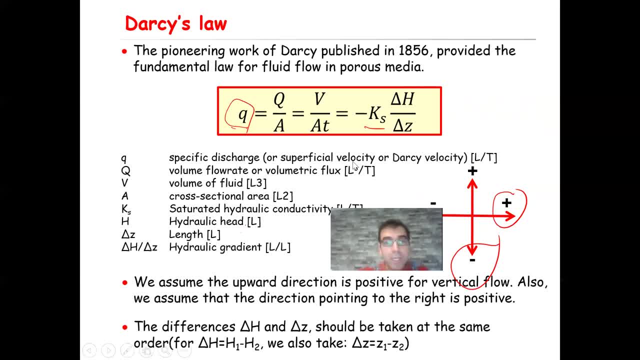 Okay, As mentioned here, I guess this one, yeah, as mentioned here. that is the dimension of length per time, like velocity, and delta H over delta. Z is dimensionless And delta H is in the unit of length. Okay,